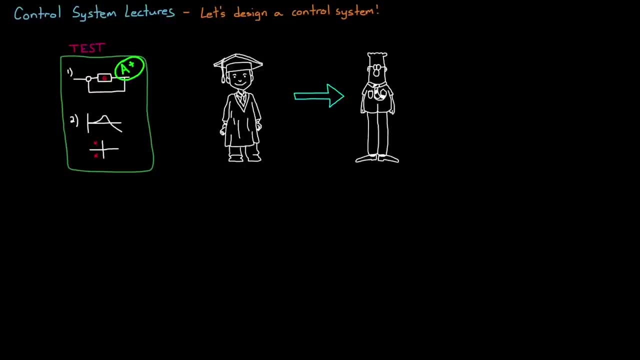 controller. I could do that, But I lacked the ability to start a problem from scratch, especially when that problem seemed nebulous and that there was more than one right answer. Where do I begin, how should I model the system, and which type of controller should I choose? 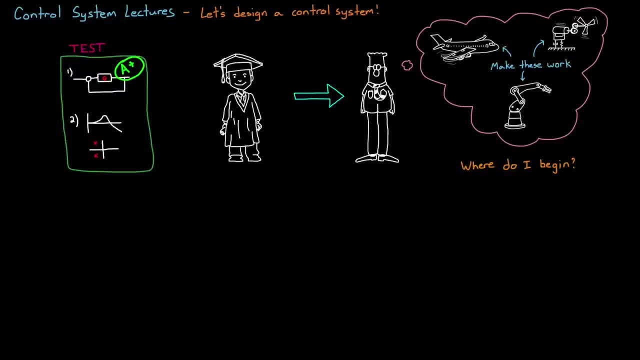 My problem came from lack of experience, for sure, But the other part came from my belief that every problem had one best solution and that I needed to know before I even started what the proper approach was going to be. I had assumed that the theory I knew was somehow. 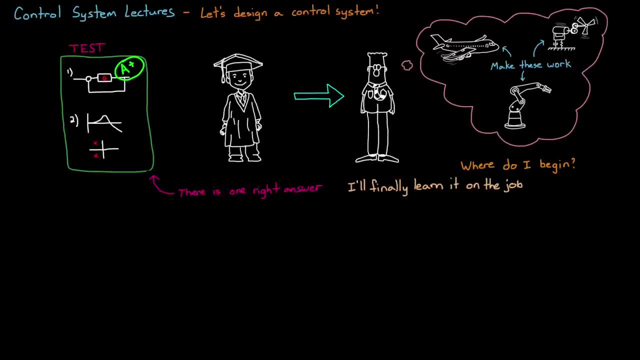 out of control because I didn't know what the proper approach was going to be. But the problem was that every problem had one best solution and that they needed to know before outdated, and I'd learn on the job exactly how people really do design, And this kept me from. 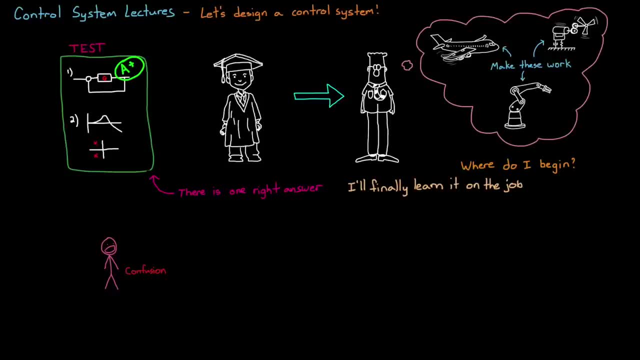 just applying the techniques that I did know to learn from it, even if it's not the optimal solution. But here's the thing: There is never a single right way to solve a control system problem. There are many different types of controllers that will produce satisfactory results. 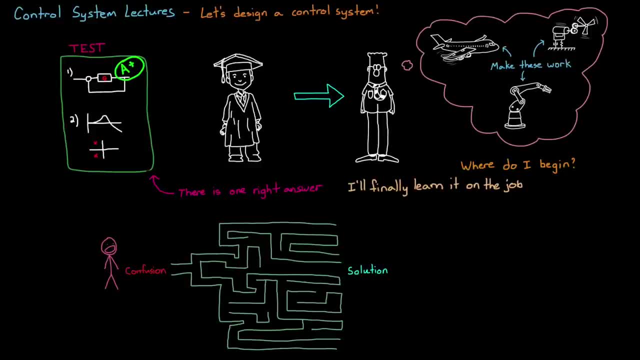 and there are numerous ways to model, test and implement that controller. If you ask four engineers, you'll probably get five opinions on how to go about designing something. Part of this is because, in addition to meeting your performance and stability requirements, there are a lot of 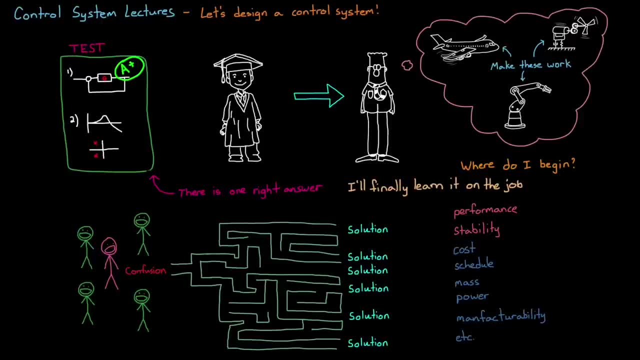 other aspects of engineering design that are just as important- Cost schedule, mass power and manufacturability, just to name a few- And a good solution must consider them as well. Often, you won't know what a good answer will look like until you jump into the problem and start exploring it. 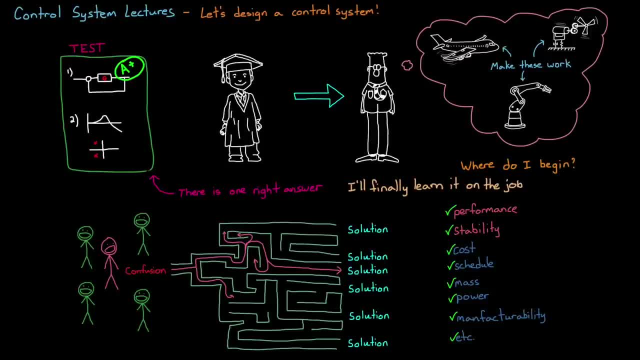 take a few wrong turns and evolve your solution over time until you're left with something that is okay. And those four engineers with five opinions might all wind up with different answers, But perfectly okay solutions as well. So keep that in mind as we walk through just a single. 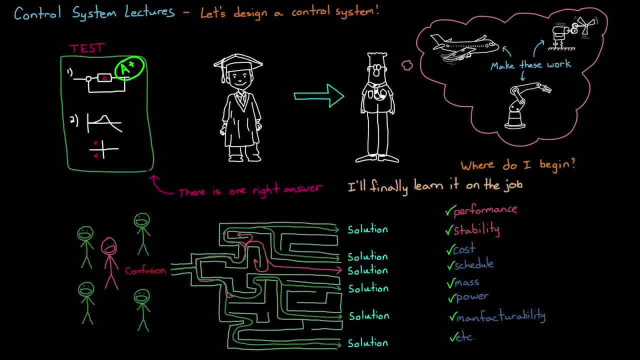 approach in this video. Now, this is going to be packed with a lot of information and it's going to be presented quickly without a whole lot of explanation. You may not be able to follow along with everything that I go through, but that's all right. It's the process and the excitement. 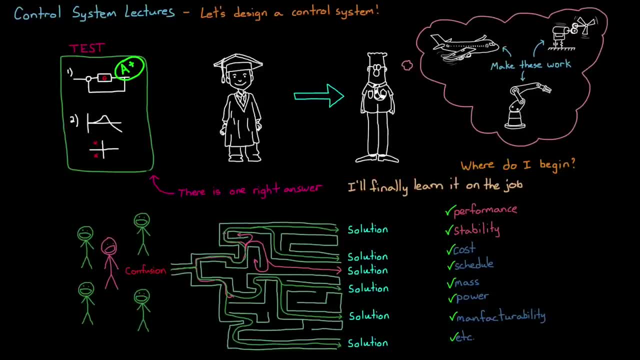 of exploring a new problem that I want you to take away from this. Hopefully this will motivate you to go off and tinker with some real hardware and practice the theory that you're learning so that you develop your own method for tackling new designs. That way, you're a little bit more. 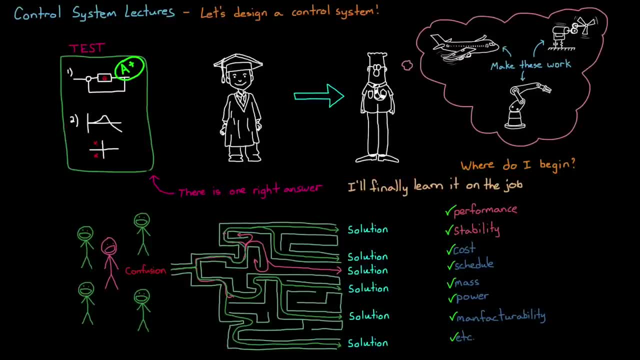 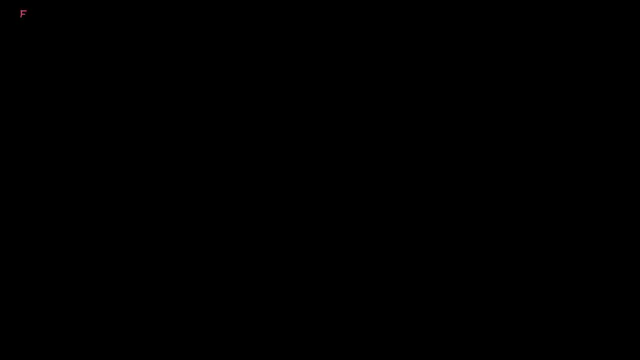 knowledgeable and at ease when you're given one of those open-ended problems at work. Okay, so with all of that out of the way, let's get to our own open-ended problem. We're part of a team that is developing an Earth-orbiting satellite, and at the moment we're 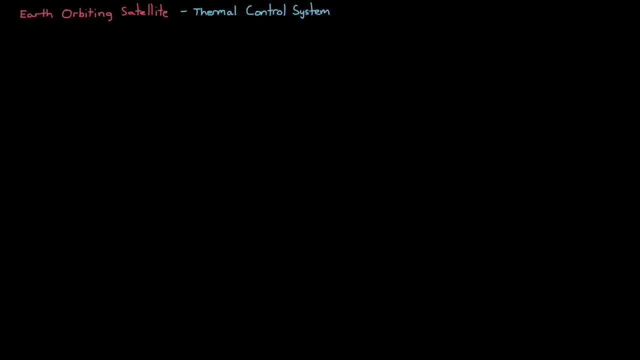 mostly concerned with the vehicle's thermal control system, That's, the system that keeps everything within the right temperature range. Space is cold and parts of the satellite that are exposed to direct sunlight are not, So we're going to be developing a new method for tackling. 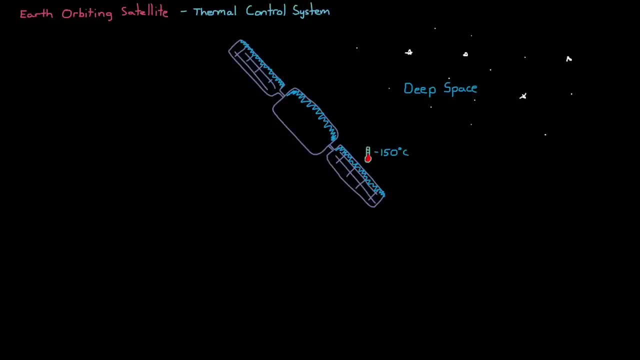 thermal control. The thermal gradient from one side of the vehicle to the other can be very extreme and changing all the time. The interior of the spacecraft is protected from these extreme temperature swings a bit because they sit within a mass that has some thermal inertia. If you look at a typical temperature plot over a 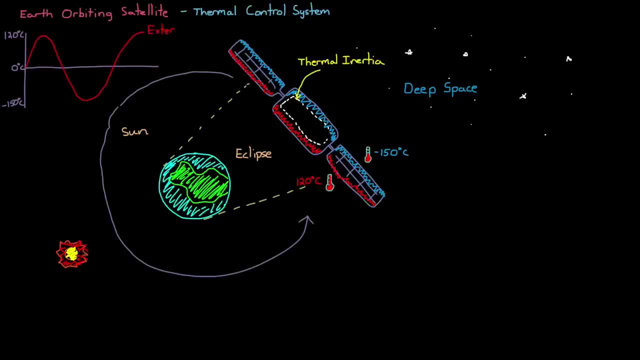 time, the external temperatures tend to swing wildly, since they're not protected, while the internal temperatures have that low-pass filter of thermal inertia, smoothing out the swings and creating a less dynamic environment. Even still, some internal components can see temperatures that are outside of their desired operating ranges, and we need to figure out a way to. 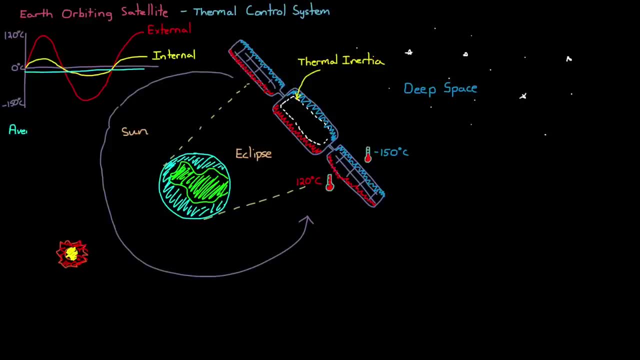 maintain their proper temperature. Let's say, for this example, that we predicted the average internal temperature for our spacecraft to be around minus five degrees C. So what does that mean for us? Well, our spacecraft has batteries, and they like to operate between ranges like zero to. 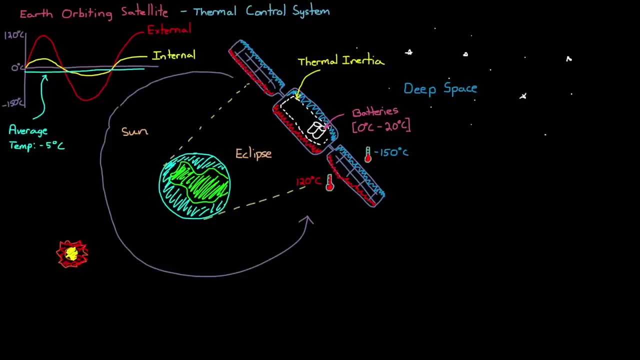 twenty degrees Celsius or so. It depends on the battery chemistry. So if it gets outside that range, the spacecraft and the entire mission could be in trouble, And our job is to develop a way to keep the batteries in this temperature range. and since we predict, 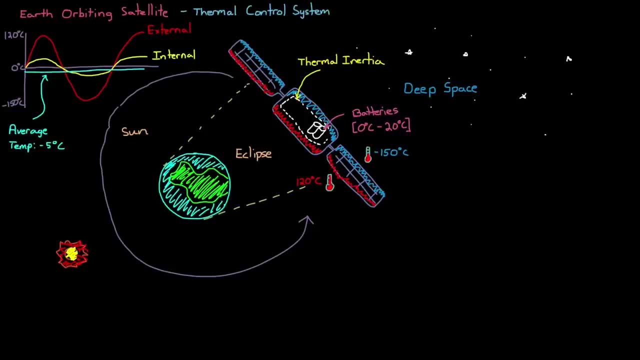 the average temperature to be rather cold. most likely we will need to warm them up rather than cool them down. A reasonable approach could be to use passive thermal control, like wrapping multi-layer insulation or an MLI blanket around it so that it traps the heat in just like a regular blanket. 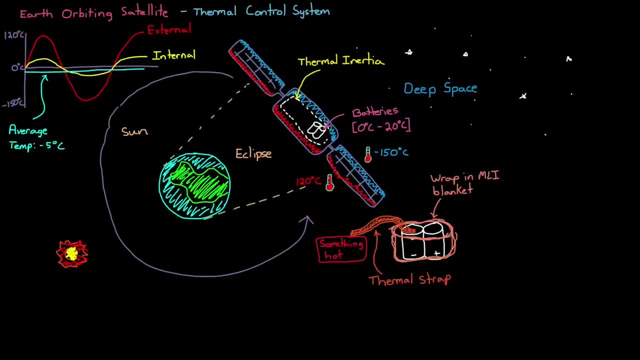 Or we could use thermal straps that connect it to another hotter component to move heat towards it. But on this particular project it was already decided for us that we would control the battery temperature with a dedicated strip heater. If you have the power to spare, 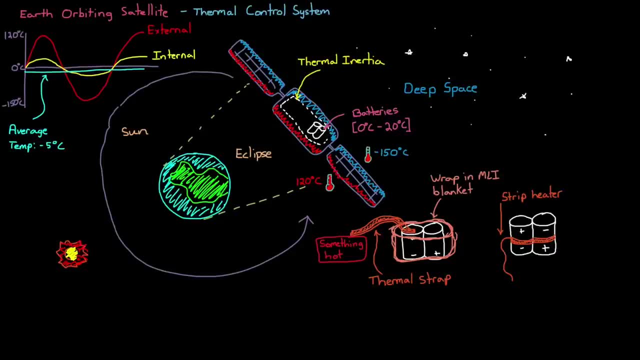 then a heater is a robust way to ensure that the lower bound temperature will not be exceeded. You have a lot more control over it with a heater and a temperature sensor bonded to the battery. So the heater, the battery, the temperature sensor and the computer that will run the. 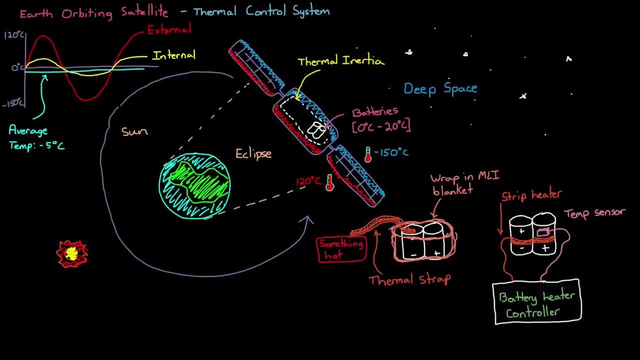 heater controller were all chosen by a different team long before we were asked to solve this problem. So we get to work with what we are given. And now that we know the nebulous problem that we've gotten ourselves into, I think for the next step it's important to understand the physics of your system, at least qualitatively. 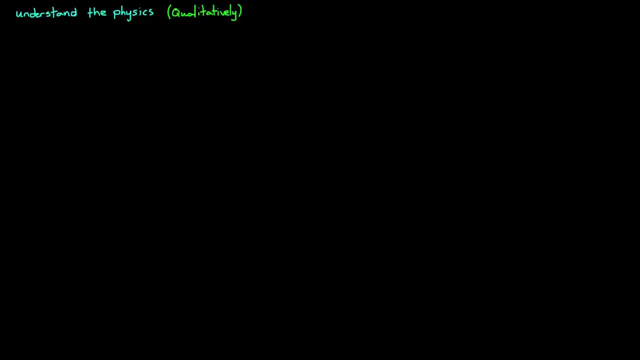 if not mathematically. before you just jump right in on crafting a control solution, I like to think about how the system can move and what it does when it's subjected to a high temperature, and how it can move around, But I'm not quite sure how it can move around. 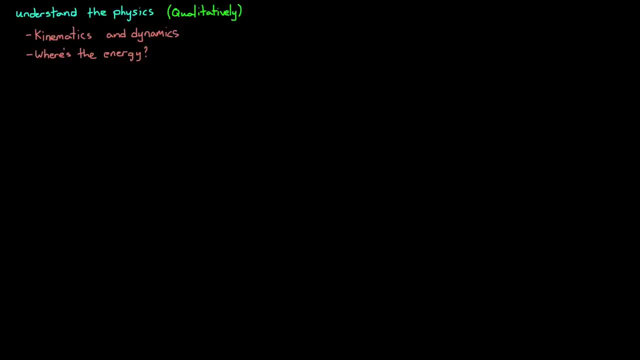 But I can't wait to see how this system can do it in the future. I'll see you next time. Thanks for watching to forces. Where does the energy come from? How is it dissipated? What are the sources of errors and disturbances in the system? I like to have this general understanding before I start, because 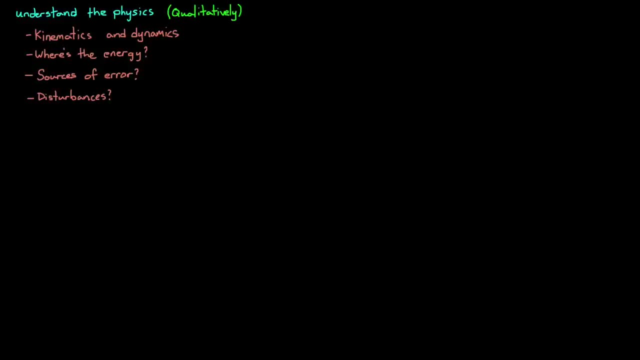 it helps guide me later on when I feel stuck on a particular problem. A thermal control system is all about heat transfer. If we think of the battery system as a closed boundary, then heat goes into that boundary and heat can leave that boundary When it's in steady state operation. the idea is: 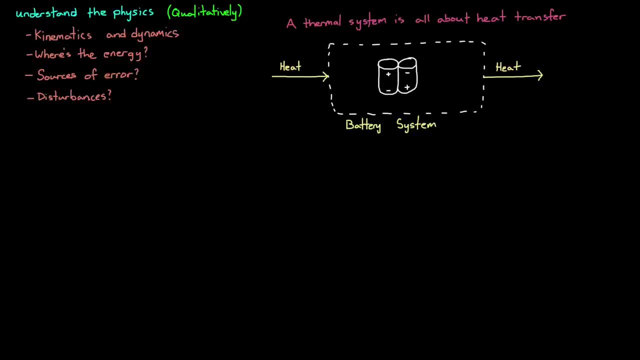 to supply the exact same amount of heat into the system that is lost out of it, so that the temperature stays the same or at least within acceptable bounds. From a simplistic standpoint, if more heat enters the boundary than leaves, the net heat transfer is into the battery system and 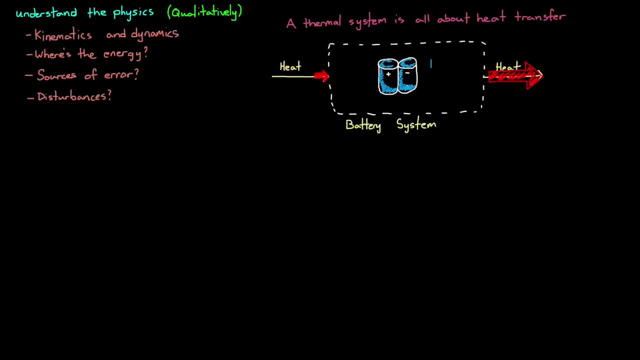 the batteries will get hotter, And the opposite is true: If more heat leaves than enters, then the battery will get colder. So what are the heat transfer mechanisms? Well, we have conduction, radiation and convection. Conduction is the flow of heat through individual particles bumping into each other and transferring 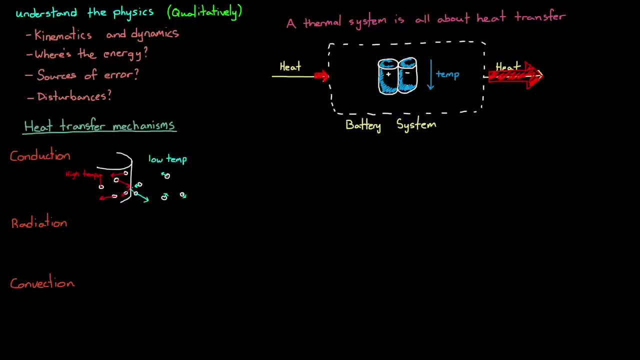 energy between them. When a high-energy or high-temperature particle bumps into a lower-energy particle, some of that energy is transferred. This type of heat transfer occurs when there is a physical interaction, like we have between the strip heater and the battery and the battery with 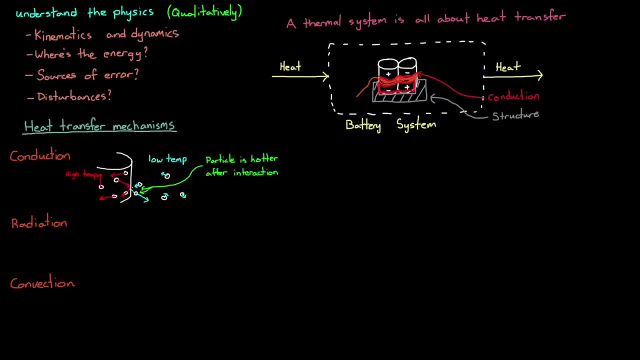 the spacecraft structure, So we need to pay attention to these physical connections. Thermal radiation is the transfer of heat through photons, or another way of putting it, through electromagnetic energy in the infrared spectrum. It's like how the predator sees things with his heat map vision. Actually, on a side note, I think it's amazing actually that every object warmer. 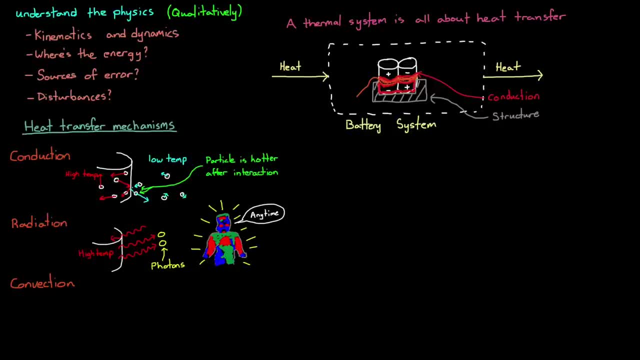 than absolute zero gives off photons. It's a crazy concept to think that humans are just light bulbs in the infrared, All right. well, our battery system emits photons also, which are absorbed by the surrounding structure, which then emits it off into the infrared spectrum. So we have a 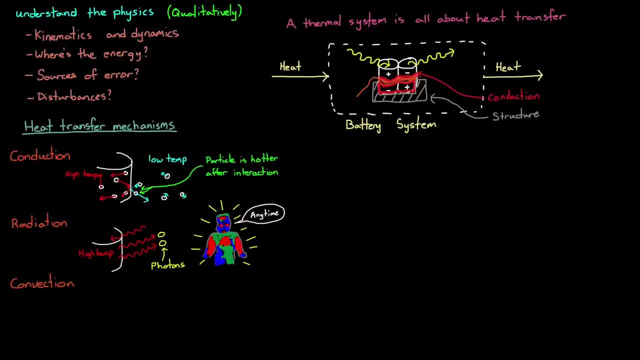 pretty crazy concept of a thermal system. So we can think of a thermal system as a particle, which is the energy transfer of a particle into deep space. Or if we're in the sun, the photons from the sun radiate into our spacecraft. 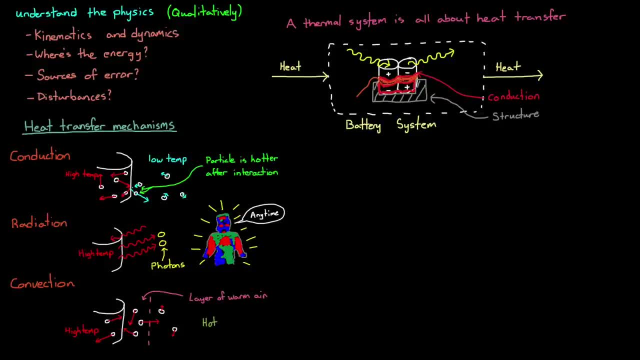 heating it up. Lastly, convection is when you physically move hotter particles out of your system, as opposed to conduction, where the particles stay and just the energy is transferred. We experience convection on Earth when the wind blows and physically moves the hot-air particles. 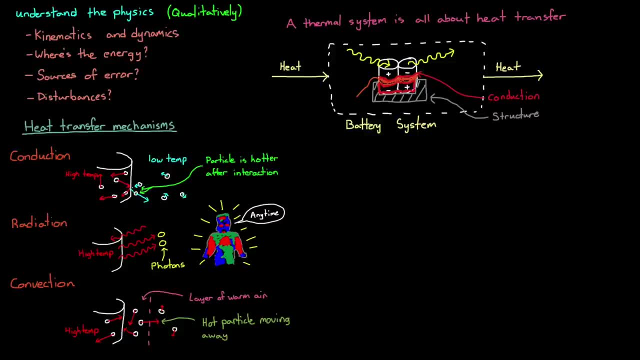 that were surrounding our body away from us, taking their thermal energy along with it. There's not a battery system, and hopefully that's obvious, So we don't have to worry about air or other bulk masses moving heat around. However, as you'll see later, we do have to deal with convection as a 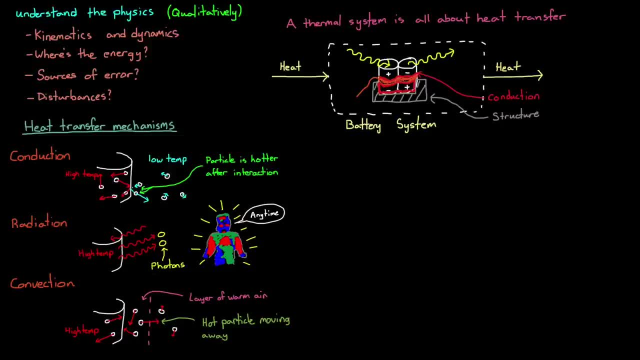 source of error when we're testing our system on Earth. Now, the heat sources for our system come from the sun, as I've already mentioned, but there's also internal heating due to the battery's internal resistance and from other hot components in the spacecraft radiating and conducting in. 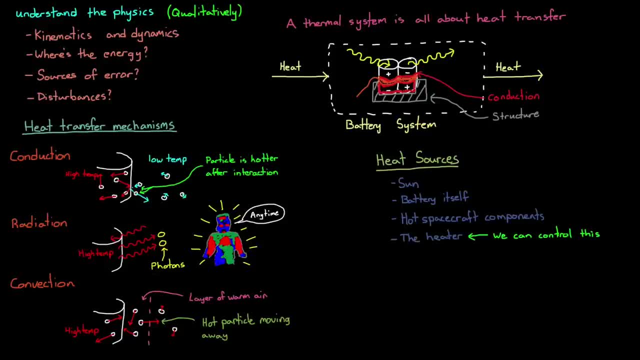 and, of course, from our heater and our heater's, the thing that we have the control over. As for error sources, there are a few, but I want to highlight just one. The temp sensors themselves will have error in the reading and, probably more importantly, they only represent a single. 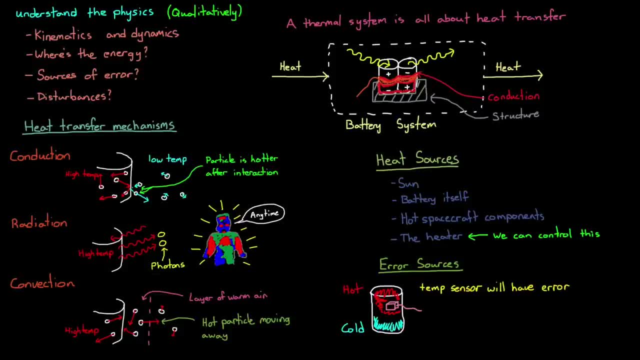 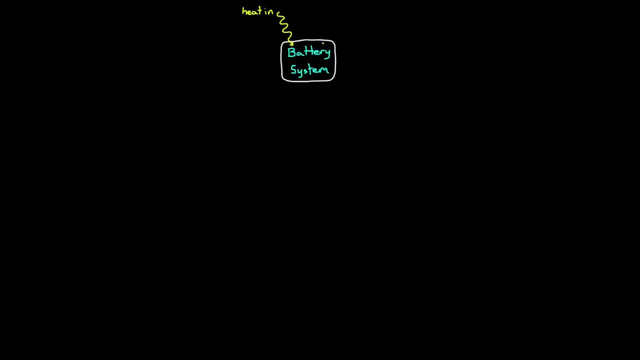 temperature point on the batteries. If the temperature isn't homogeneous, we may have problems with part of the battery getting too hot or too cold, and our sensor not being in the right spot to measure it. So where should we go from here? Well, if we knew the battery system perfectly. that is, how much heat enters and leaves the system. 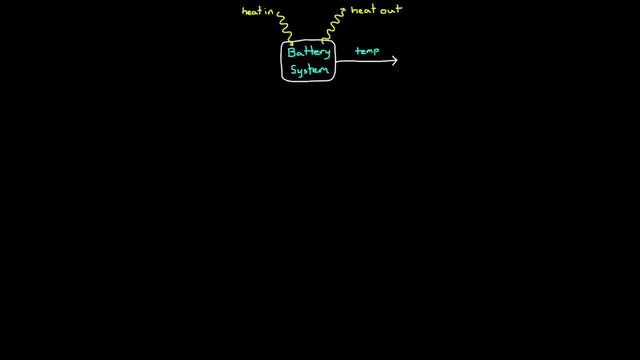 while on orbit and we knew how the delta heat changed the temperature of the battery system, then we could just set the heater to the proper supply value to make up the difference and be done. This is an open-loop control design because the heater set point doesn't rely on feeding back. 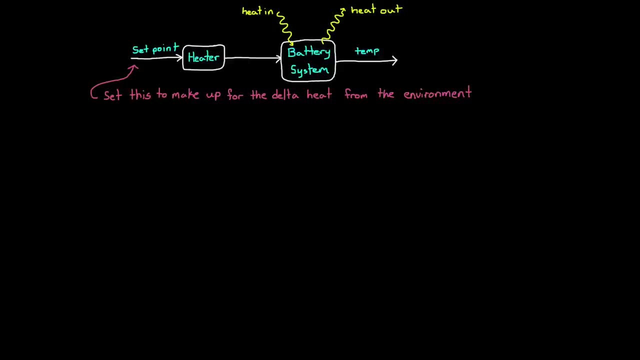 the battery temperature. With this design. if we're wrong about the outgoing or incoming thermal energy, then the battery temperature will be off from what we desire and the controller will have no way to compensate for that error. It's a predetermined set point. 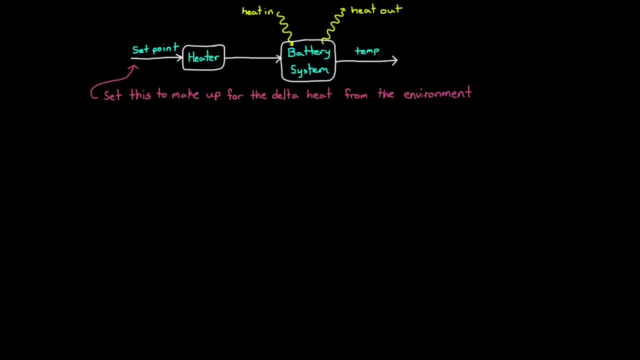 Now, this might be a good approach if the system was going to operate in a well-controlled environment. However, that is not space, because the external environment is always changing. We have different spacecraft components that are being turned on and off. there's eclipse as it. 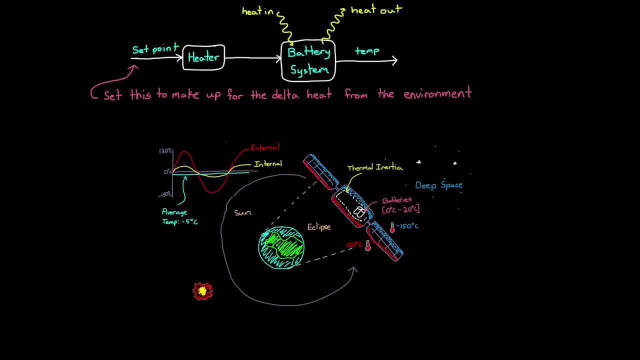 orbits and different spacecraft rotations to take into account. Even the sun's output changes over time. No, the open-loop approach feels risky for a control system like this. So if we were to use a critical spacecraft component, because I don't have confidence that we can predict the 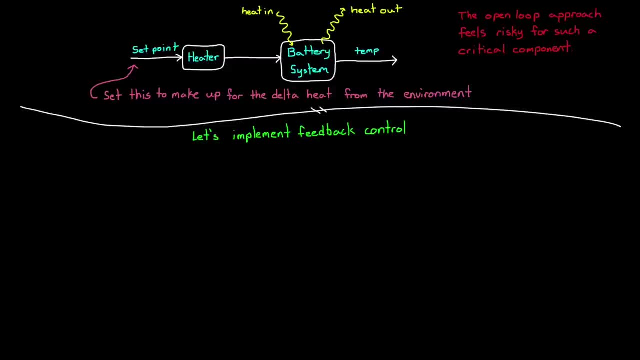 environment that well. so we should implement feedback control, at least of some type. We need something that determines the heater set point, based on the actual temperature of the battery system, something that feeds back the temperature. In order to do that, we need a 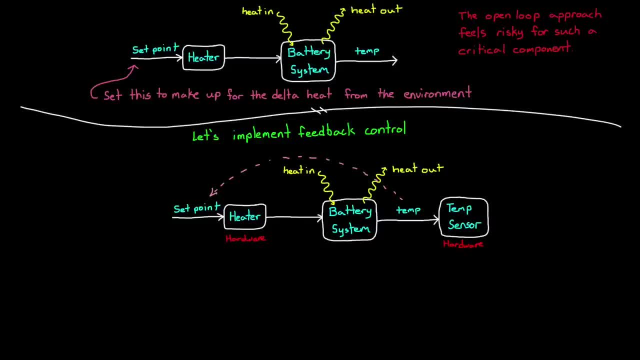 temperature sensor. Now, the temp sensor, the heater and the battery system are all hardware components. To get to where we can develop a software-based controller, we need some kind of sensor manager that can read and interpret the voltage from the sensor and produce a meaningful 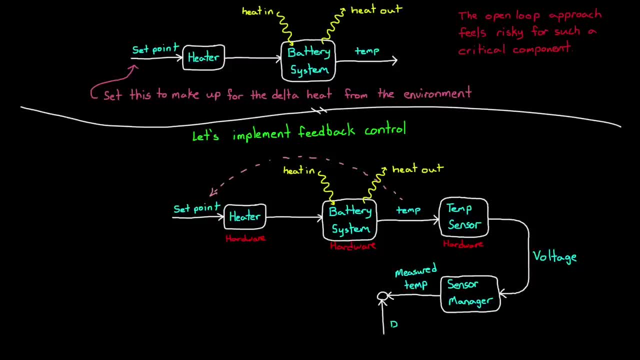 measure. Now with this measured temperature we can subtract it from our desired temperature to get an error term or how far off our actual temperature is from the desired temperature. For example, if we wanted the battery to be at 10 degrees C but it was measured to be minus 5. 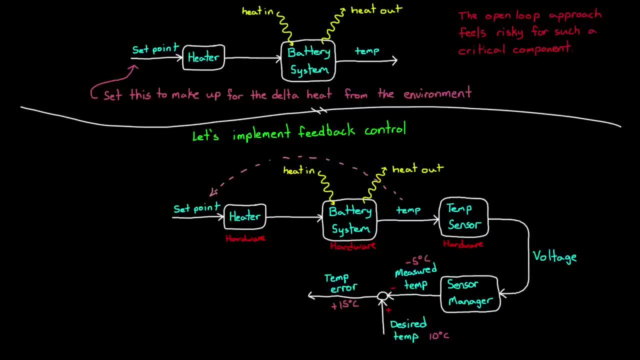 degrees C, then there would be a plus 15 degree difference and we would need our heater to supply more heat. This is fed into a controller that takes that error and tries to calculate the right heater set point. When we're developing a controller, we're trying to determine how that. 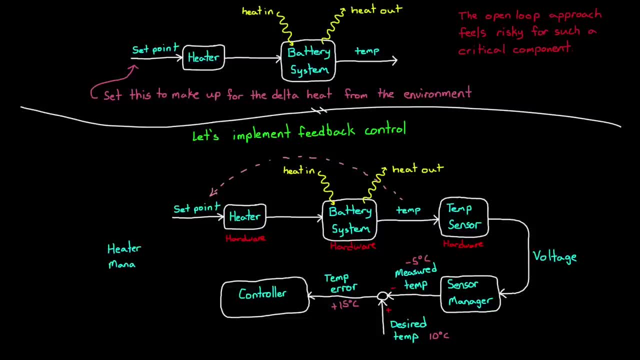 conversion is done and the output of that controller would go into a heat manager, which would generate the voltage needed to drive the heater. All right, now that we've connected the battery temperature back to the heater set point, we have the framework for our feedback control. 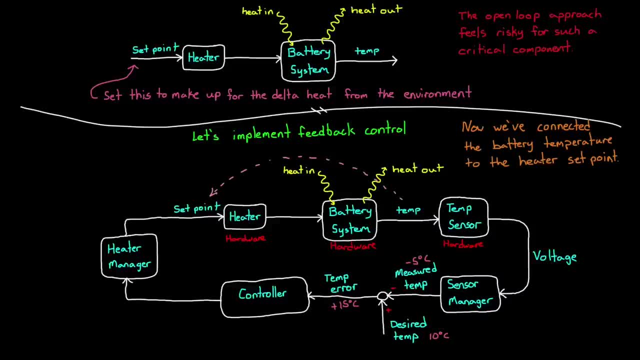 system. But now what? Well, unfortunately, we weren't given any transfer functions for the heater, the battery system or the temperature sensor, and I don't want to create a control law without knowing a bit more about what's going on in the system. So let's get started. 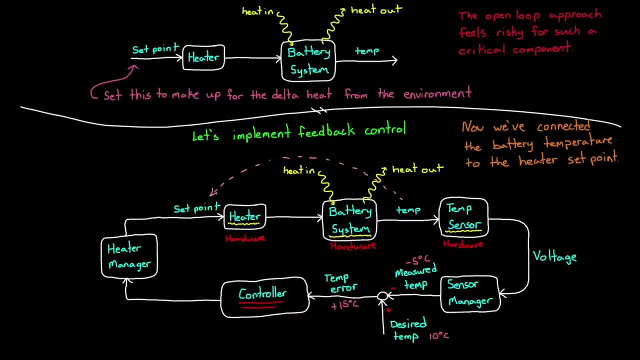 For example, it's important to know how the system will behave when subjected to actuator commands, or, in this case, what does it do when we turn on the heat? If we don't have that, it seems a bit like shooting in the dark. And to proceed, we need to know more about the physical hardware. 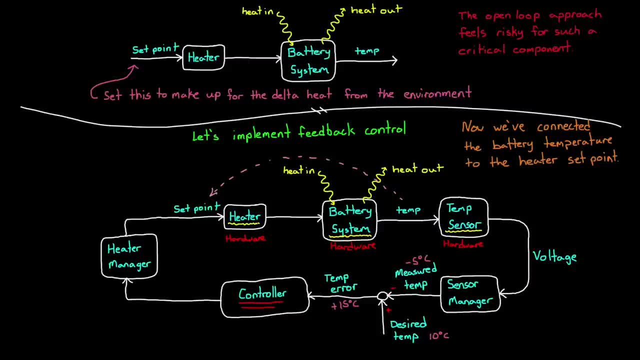 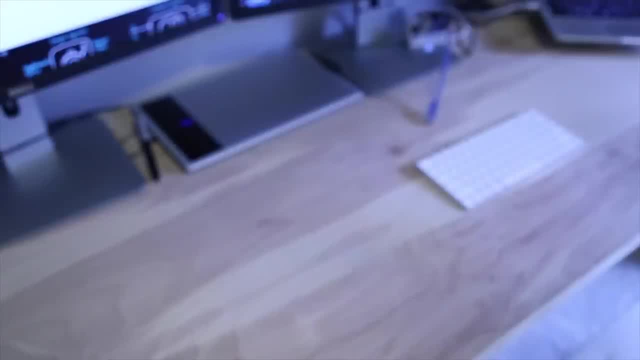 and luckily we do have access to a physical test bed with real flight components, So let's play around with those and see what we can learn In this video. the hardware I'll be using is this temperature control lab, which runs on an. 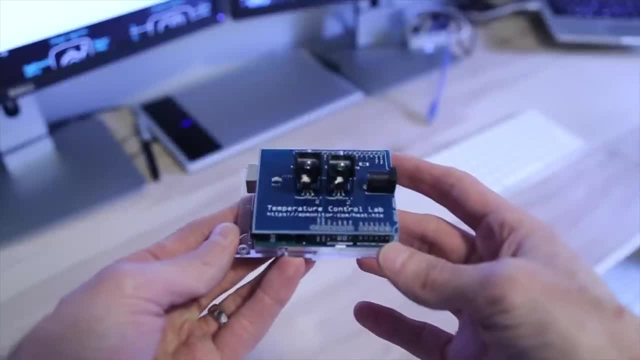 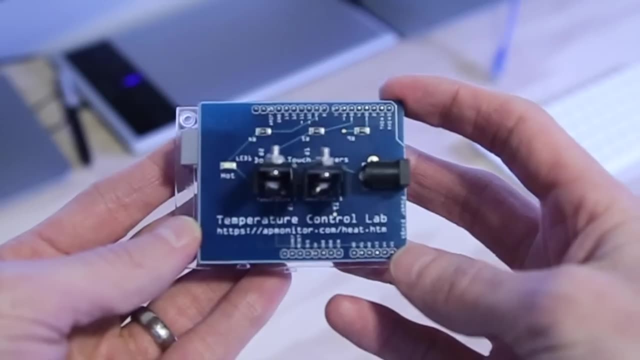 Arduino microcontroller. Clearly this is not real spacecraft flight components, but for this video it will still do just fine, because it has heaters, sensors, thermal mass and a computer, just like our problem. We'll be able to learn a lot from operating this hardware, but to tie it. 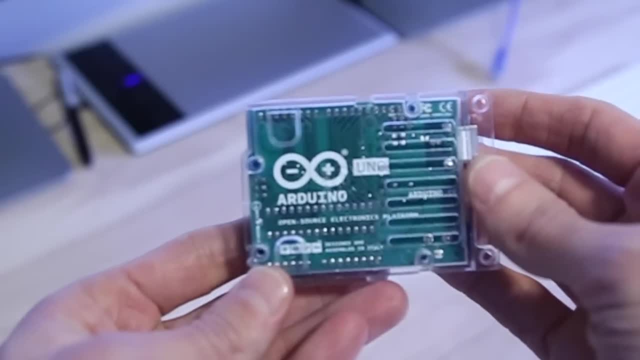 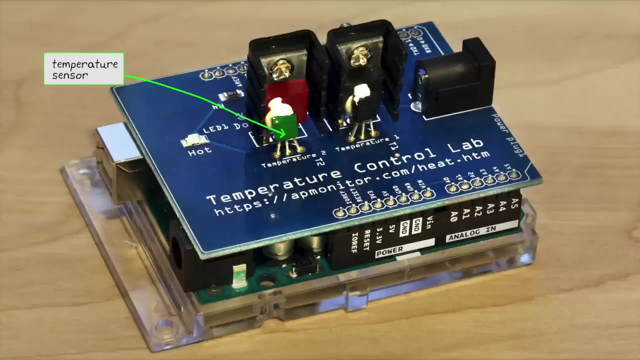 back to our spacecraft. you'll just need to use a little imagination. Let's walk through it in more detail. There are two sets of heaters and temp sensors, but we're just going to use a single one for our test. The temp sensor is highlighted in green and it's bonded to the temperature sensor. 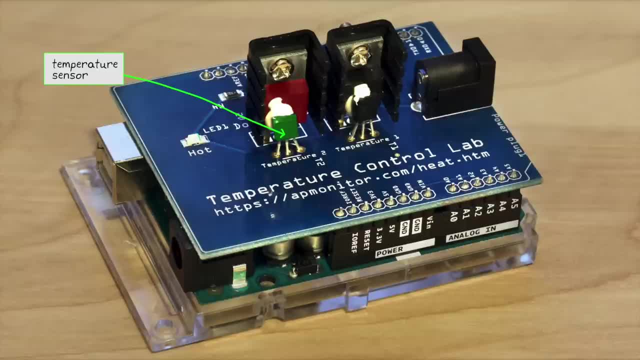 The temp sensor is highlighted in red with white thermal epoxy in between the two. The thermal epoxy creates a good conductive path between the heater and the sensor. Surrounding the heater is a radiator that helps distribute the heat and gives the system a bit of thermal mass There. 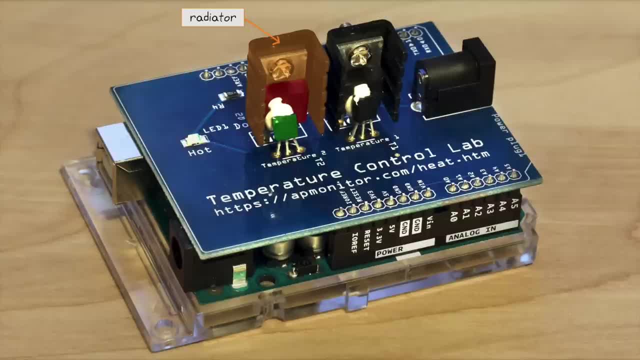 are no physical batteries in this test hardware. However, these radiators will serve the same purpose. They are a thermal mass that we can heat up and, when hot, they lose heat to their environment. The heaters are controlled by, and the sensors are read by the microcontroller. 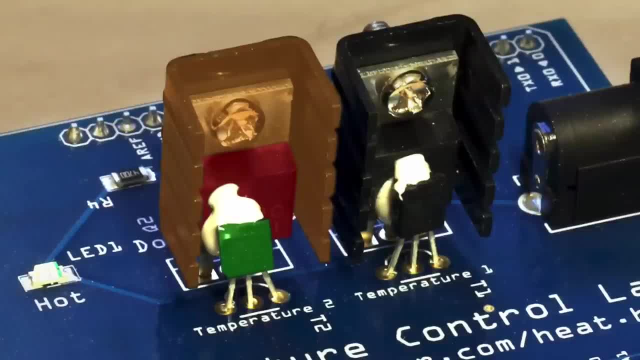 underneath. Now this setup provides several ways for the heat to get to the sensor. There's a conductive path through the epoxy and another weaker conductive path down through the copper in the board and back up through the sensor's pins, And we have some thermal radiation coming. 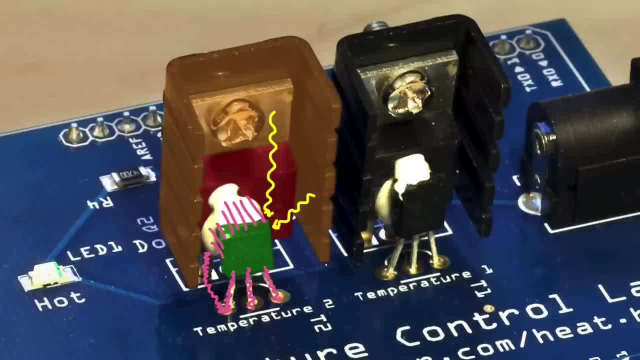 in from the aptly named radiator, And we also have some convection heat transfer due to the moving air. We shouldn't need to worry too much about the impact of convection, because the conductive path through the epoxy should dominate. When you're running a test, you should take note of how that test differs from the real operating. 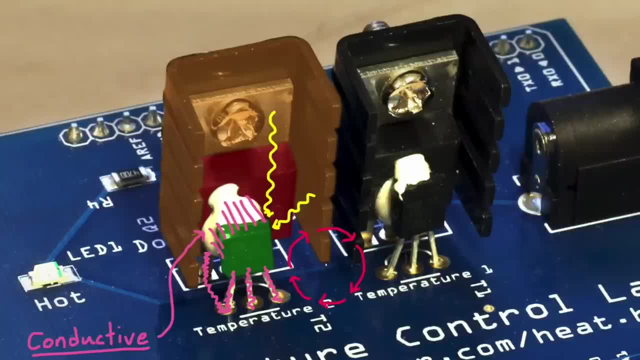 environment. It would be a shame to design a control system that could perfectly control your test bed, only to find out later that the real hardware in the real operating environment doesn't behave the same way. Now there's a lot of differences in my test setup, However. 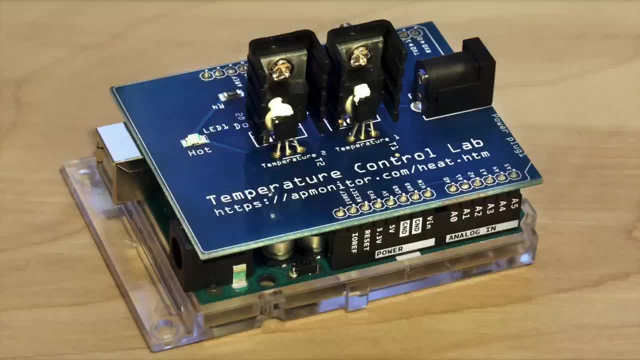 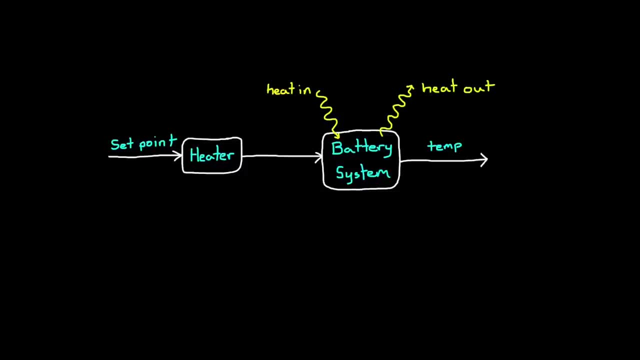 I want to highlight a few important ones. I already mentioned that there's no air convection in space, But another is that we don't have the rest of the satellite which can radiate heat to or from our system. And finally, the ambient temperature is a little bit different. The ambient temperature. 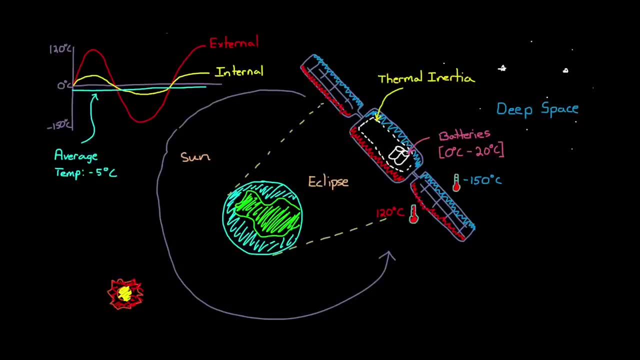 is not minus 5 degrees. I don't think my AC can go that cold. So with these differences the dynamics of our test will definitely be off. But we can still learn a lot from a physical test like this if we set up our control system well. 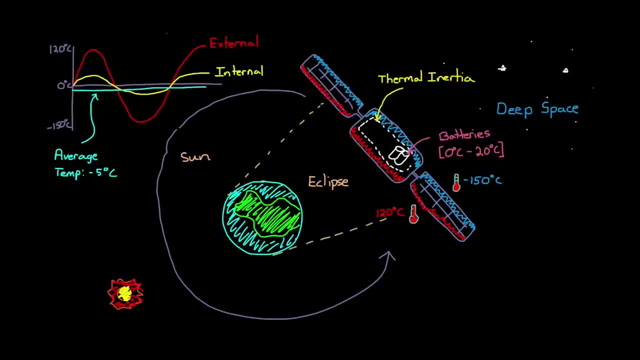 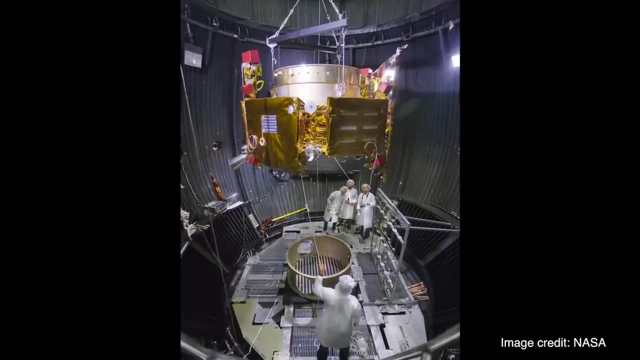 We can then tune and configure it with simple software commands later on. This difficulty in having a representative test environment is why, even after everything has been designed and built, a spacecraft will still go into a giant thermal vacuum chamber and test all of its components in a more space-like environment. 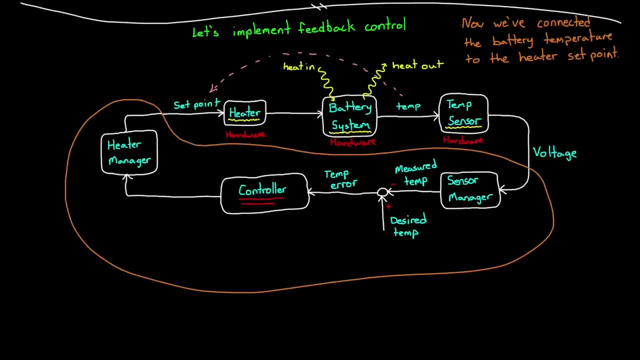 If we go back to the block diagram, everything I'm circling in orange would normally run on the Battery Control Processor or the Arduino. in our test, However, rather than attempting to design and tweak a controller on the Target Processor, it'll be easier for us to do all. 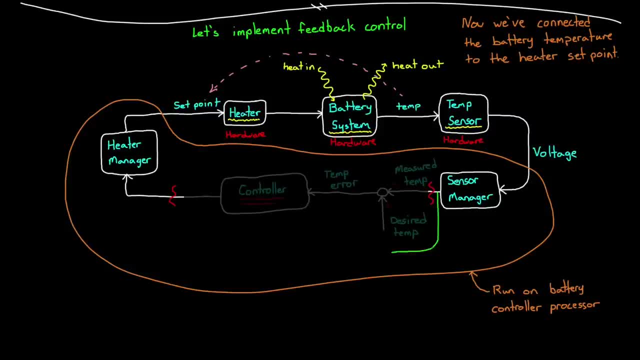 of the design work using a program like MATLAB or Python. The Arduino will still be responsible for managing the heater and sensor devices, but will send the temperature back to my main computer, run the control law there and then send the heater commands back to the test hardware. 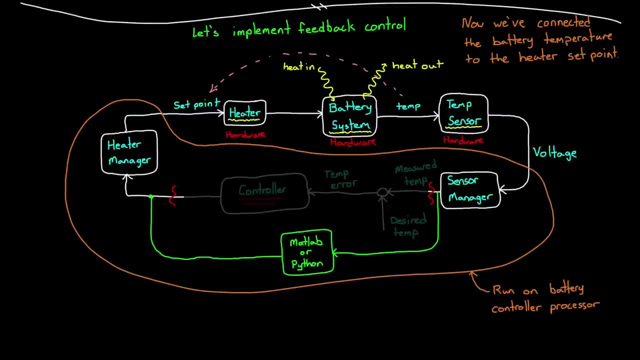 And then, once we're satisfied with our controller design, then we can load our controller code onto the spacecraft and have it run for real. This type of testing is called hardware in the loop because, rather than simulating the entire system with mathematical models, some parts of the system, like the sensors, actuators, 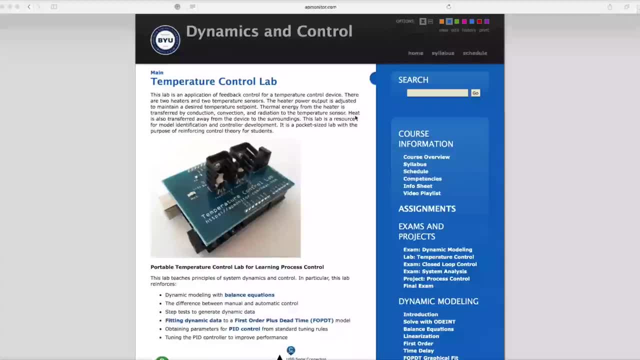 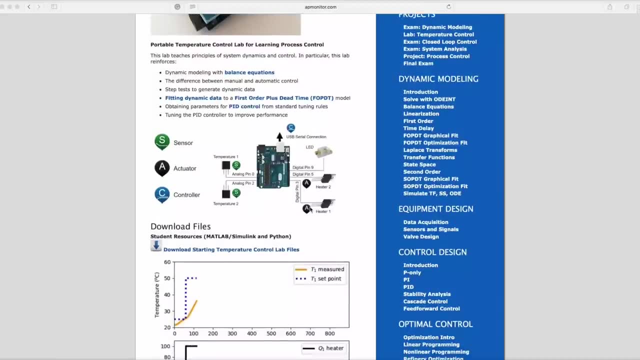 and thermal mass are real physical hardware. Getting the software for this test to run is easy because the temperature control lab comes with all of those files. If we go to apmonitorcom, slash heat dot htm, we can download the device manager and the 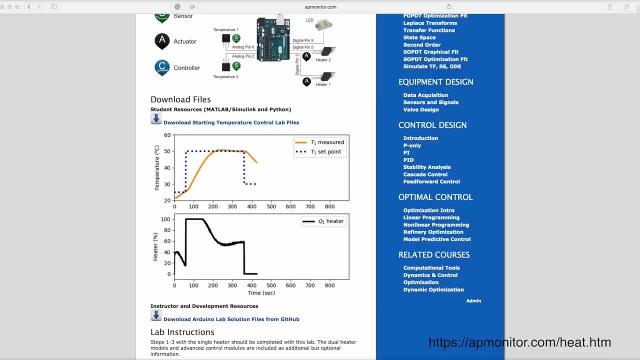 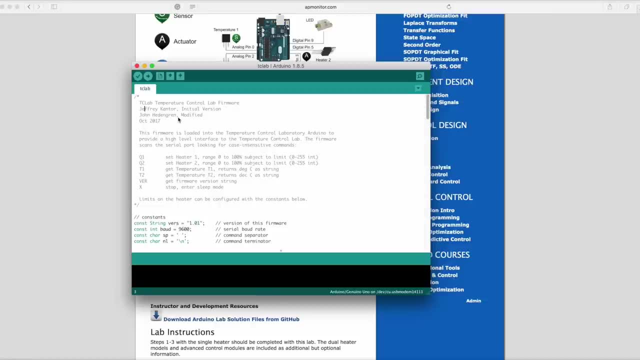 code that will allow your computer to talk to the hardware using either MATLAB or Python. It's your choice. The device manager is the tclabino file that will load directly onto the arduino, And this file defines which pins the heaters and sensors are connected to. reads and writes. 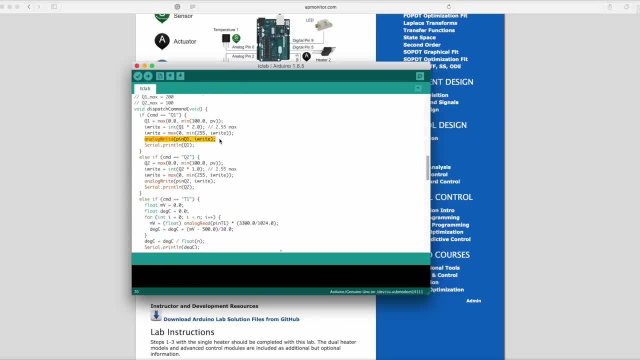 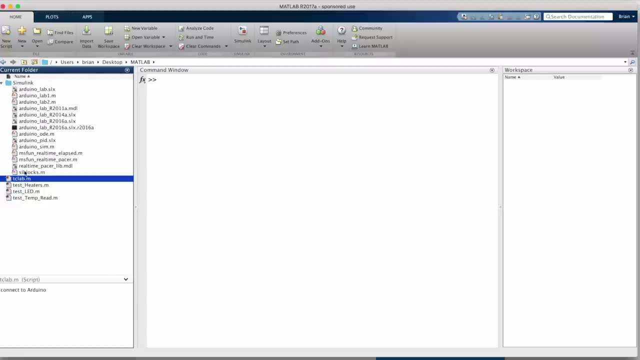 to those pins and interprets commands from my computer. Now I'm using MATLAB. I'm using MATLAB for the interface because I think Simulink provides a better visual for what we're doing here and I think it's easier for you guys to follow along. 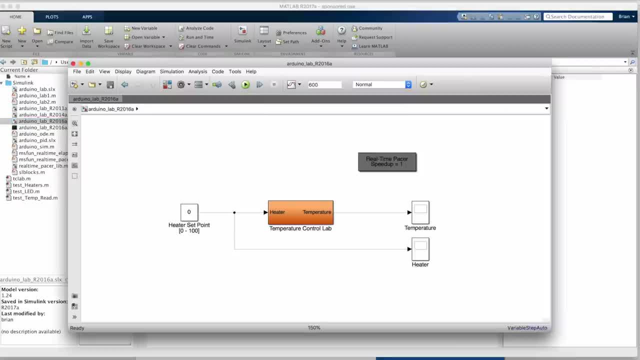 I'll open the Simulink file and show a very basic system. The orange block is the software that communicates with the test hardware. You can think of this block as the physical hardware sitting on my desk. If I send a heater command to it, it will physically turn on the heater. 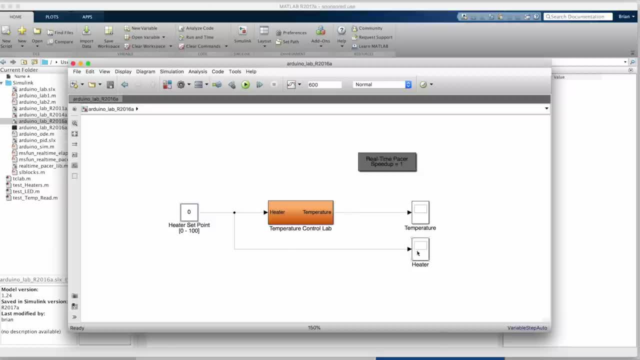 Now I can set the heater between 0 and 100 percent and get the resulting temperature back from the hardware. This gray box ensures that when I run this test it will run at real time speed, And at this point I just need to hook up the hardware to my computer so it can talk over. 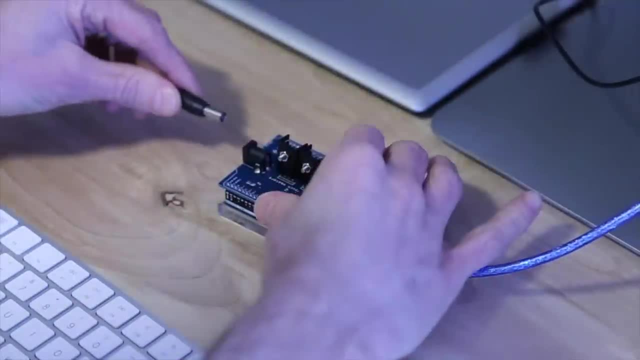 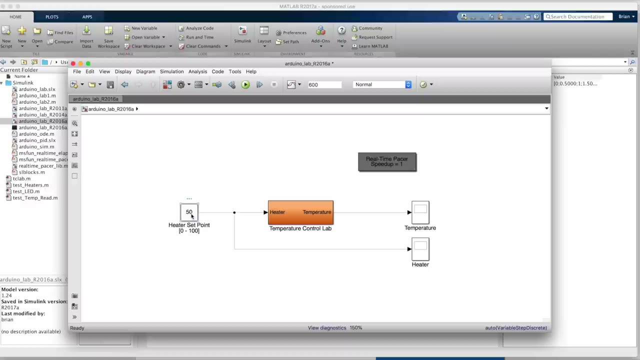 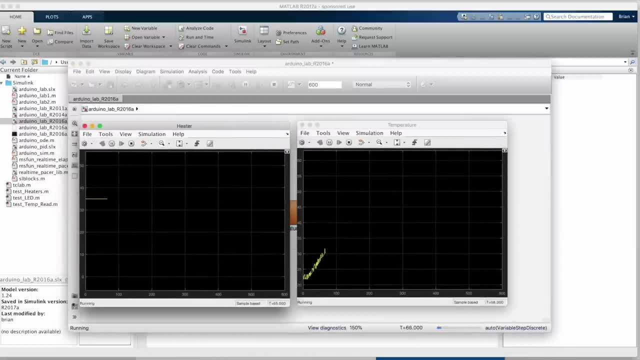 I'm going to run the test. I'm going to run the test Now. temperature doesn't change that quickly, so I ended up running this for about 10 minutes. I'll speed it up and spare you the time. Notice the shape of this response. 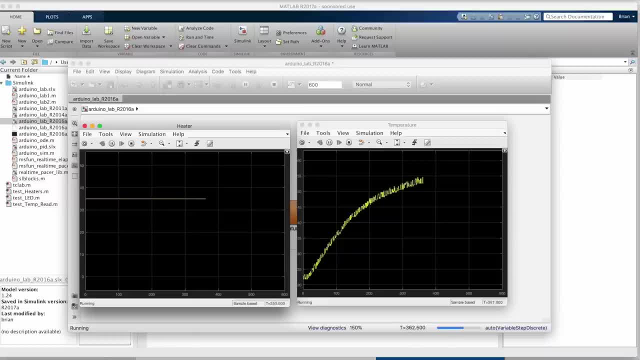 It increases quickly at first and then tapers off to about 55 degrees by the end. If we were trying to hold the temperature at 40 degrees, this would be too high. We'd have to lower the heat point by some amount. But remember, open loop isn't the solution we're going for. 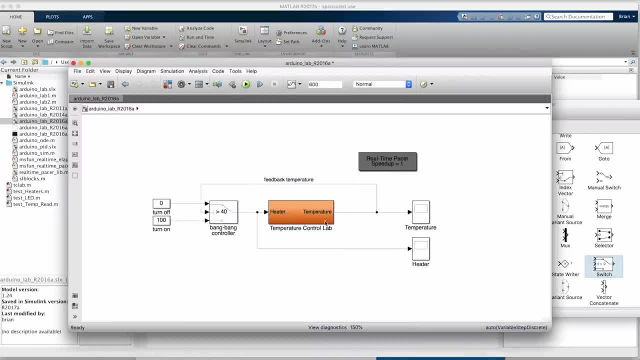 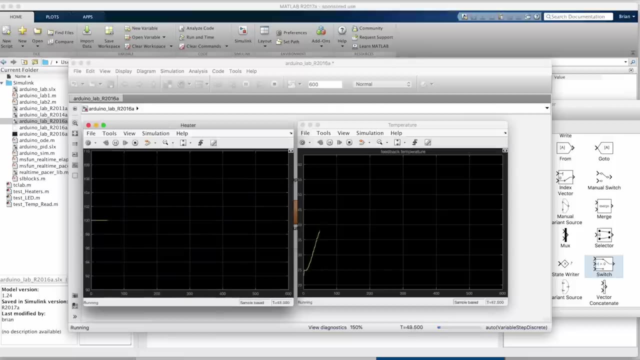 So let's change our system to be closed loop. For my first attempt, I'm going to create a bang bang controller. This is a very simple non-linear controller that will turn the heat on at 100% if the temperature is below 40 degrees and turn the heater completely off if it gets above 40.. 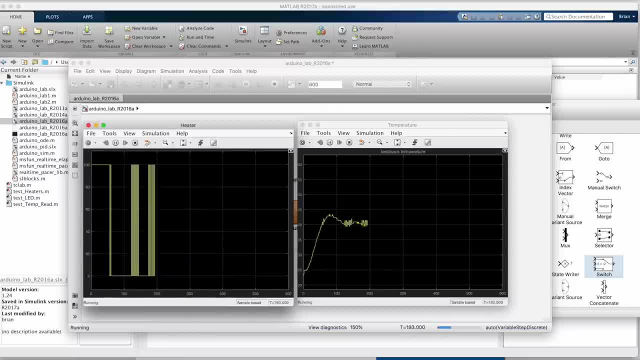 Let's run this controller and see how it does. Again, I'll speed it up. Okay, let me pause it here. Look what happened with this controller. The temperature rose faster this time since the heater was on full blast, but it overshot. 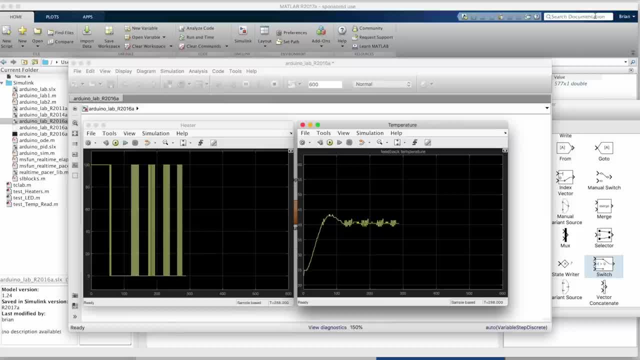 40 degrees before starting. We're settling back down and hovering around our set point. Why would this controller overshoot? It doesn't make sense that the temperature would continue to get hotter after we stop supplying heat, right? Well, the heater will stop getting hotter. 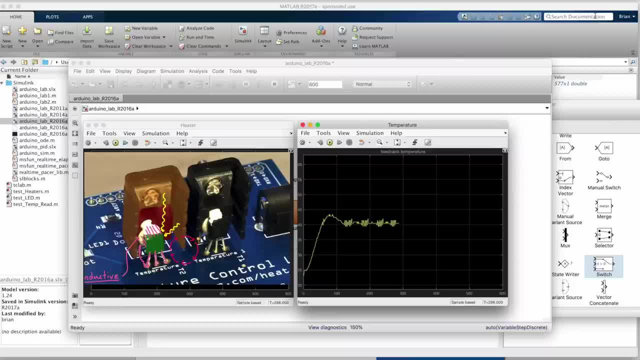 The problem is that there's a delay between the heater getting hot and the temp sensor sensing it. The heat has to flow through the thermal epoxy, and so the heater was actually much hotter than 40 degrees when we turned it off, and that extra temperature caused heat to still. 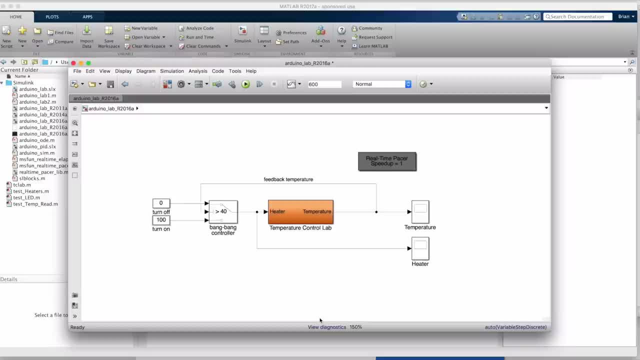 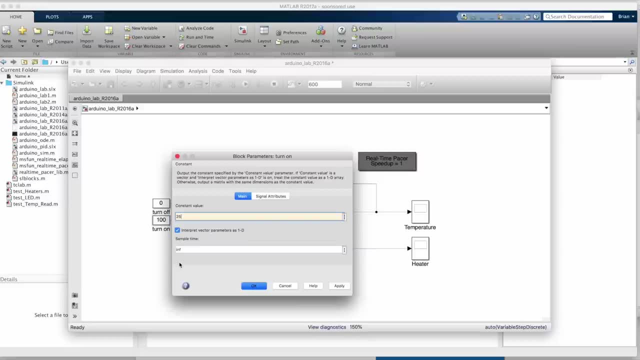 conduct to the sensor after we turned it off. So we're going to have to wait a little longer for the temperature to go down, And I don't like that overshoot. so let's see how to get around it. Let's just change the heater set point to 25% when it's on, rather than 100%. 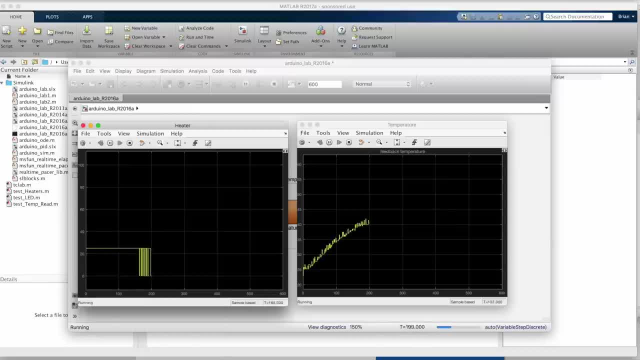 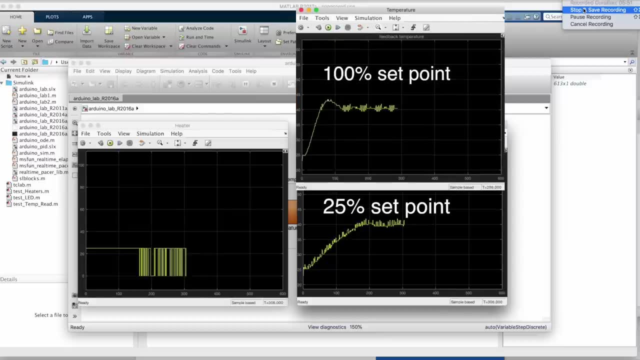 This should reduce how hot the heater gets and lower the overshoot after we turn it off. And look at that: No overshoot. But now we've introduced a new problem because the temperature doesn't rise as fast with this lower set point and we need it to be able to respond quickly to the changing thermal. 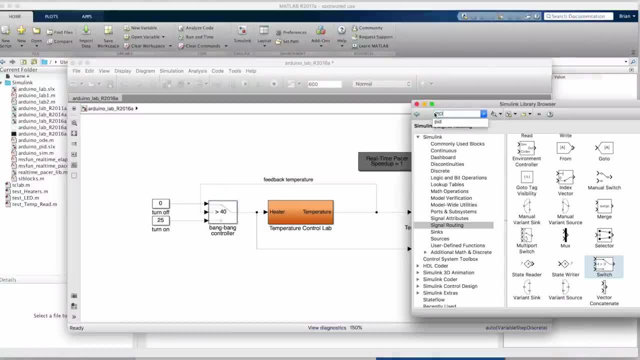 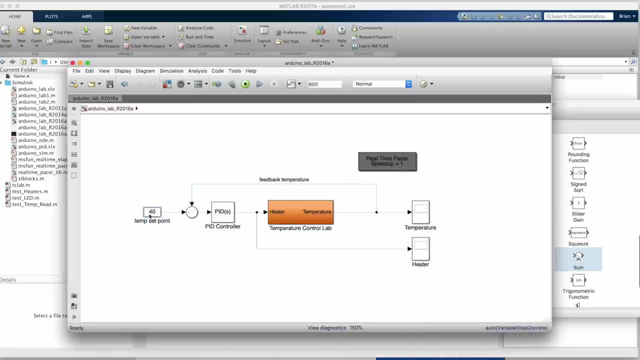 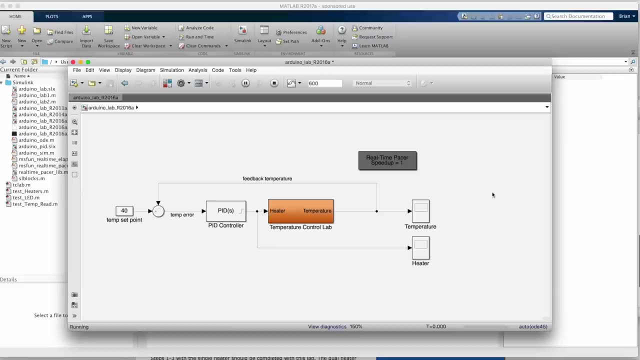 environment. so this won't do either. We need a controller that can set the heater high at first to heat up quickly, but back off earlier to slow the rising temperature before we overshoot, And we can do that with a PID controller. I'm using the built-in PID controller with Simulink and I set the P, I and D parameters. 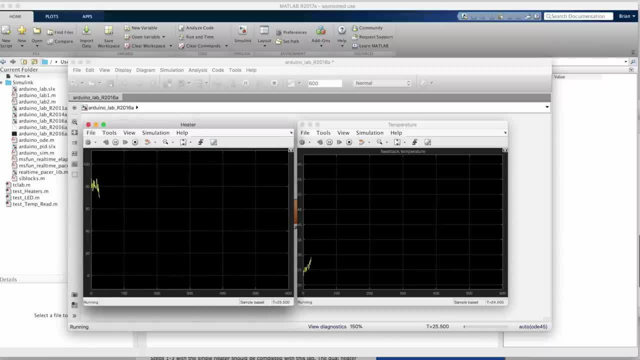 to a first guess And if I run this, you'll notice a few differences from the Bang Bang controller. First, the heater set point on the left is no longer jumping between a max and min value, but is being set to a continuous set of values. 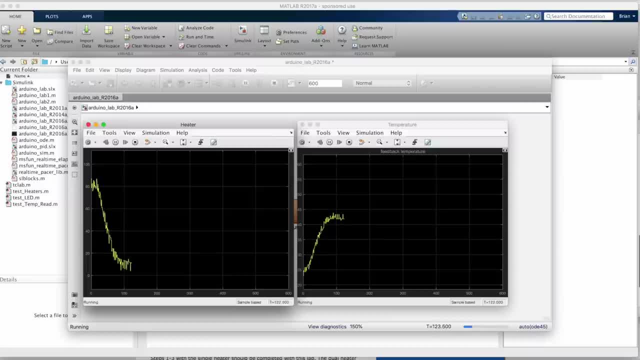 And that's because the PID set point on the left is no longer jumping between a max and min value, but is being set to a continuous set of values, High at first when we want the temperature to rise quickly and then lower as it reaches. 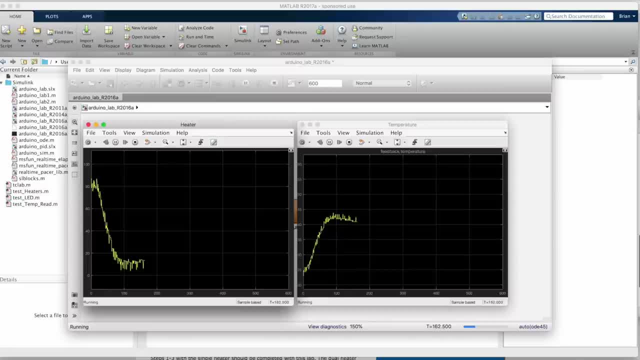 its desired temperature. Now there's still an overshoot, which means I don't have it tuned very well. I could probably increase the D term to remove the overshoot. However, there's something else that I want you to notice. When the temperature is steady at 40 degrees- we can see the heater set point is steady. 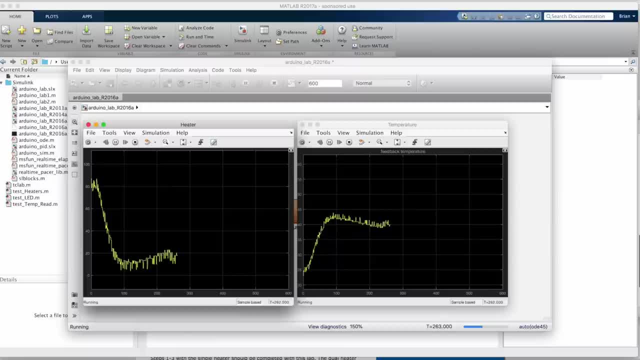 at around 17%. This means that the heat that is supplied at 17% is exactly the amount of heat that is lost to the surrounding environment portion that our heater makes up. So you might be tempted to just go back to our open loop system. 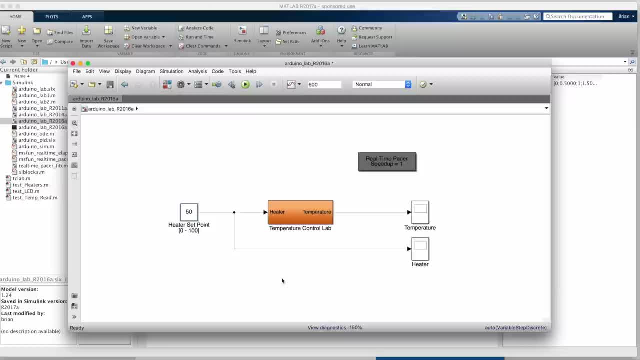 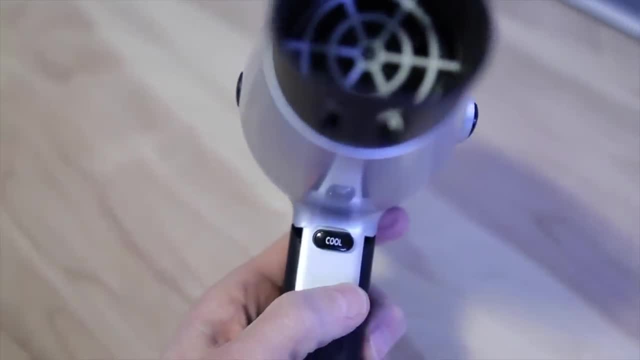 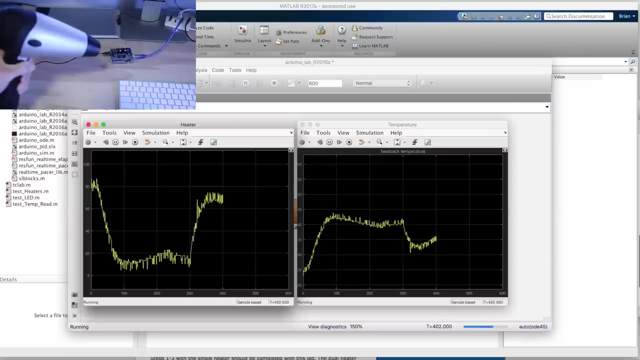 and set the heater to 17% and be done. However, this will only work if the environment stays the same. Watch what happens when I remove more heat with a hair dryer set to cool: The temperature immediately drops and the PID controller rises the set point to counteract it. Eventually, the 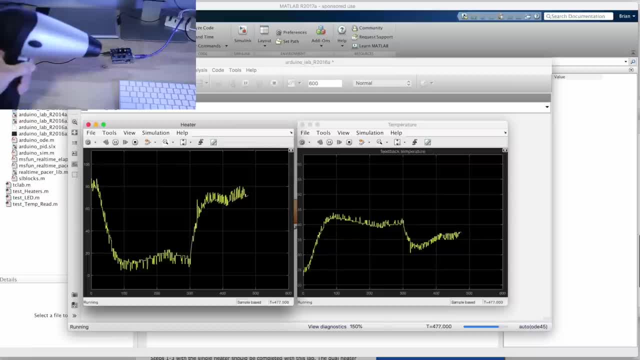 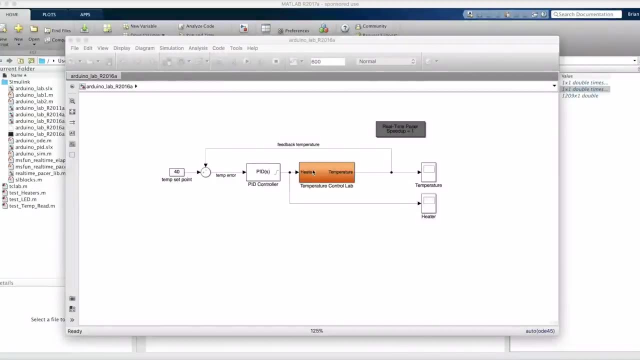 temperature gets back to 40 degrees. but now you can see, with this changed environment, the heater set point settles at around 75% and not 17%. This is reinforcing that we really do need this feedback controller. Okay, at this point I could go back and tweak the PID gains and see if we can. 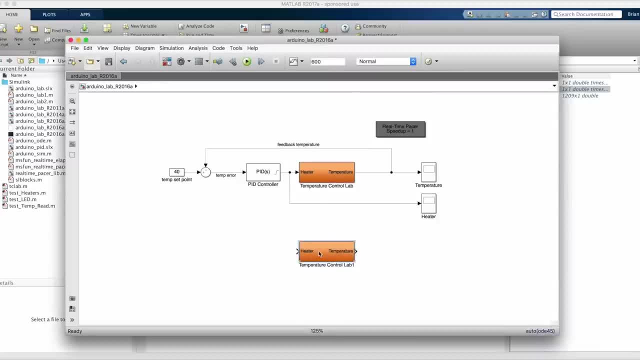 get a better controller, but it takes 10 minutes every time I run this, and this is taking a long time. Not only that, but most of the controller designs that I want to try require me to have a mathematical model of the system, which I don't have. We've done everything so far without really 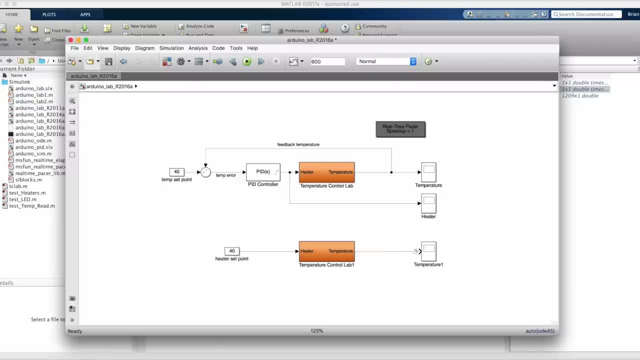 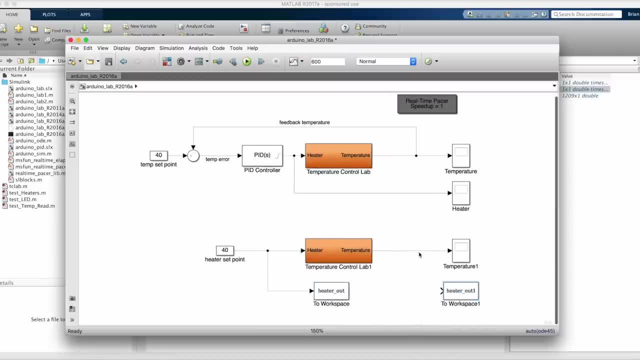 knowing anything about our hardware. So at this point I want to do some system identification. For system identification, we could take the white box approach, taking note of the material properties and the dimensions, and write out the differential equations directly. However, we have the hardware, so let's fit a transfer. 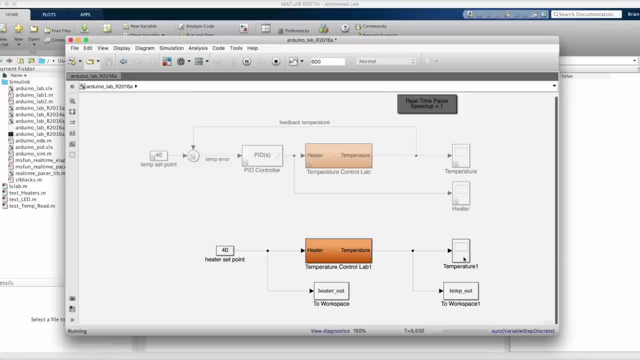 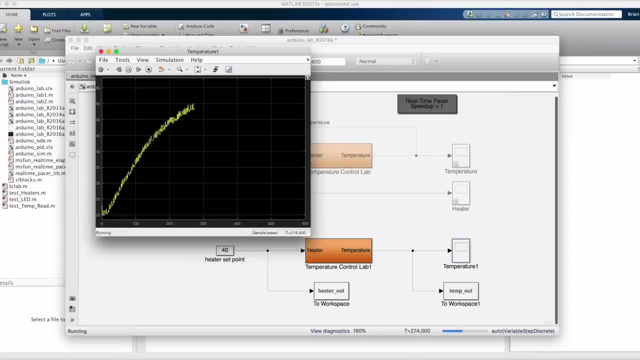 function to our real system. The way I'm going to do that is by applying a step function to our system and recording the step response. This is exactly what we did at the beginning of all of this, except this time I'm going to save the data in an array to use later. 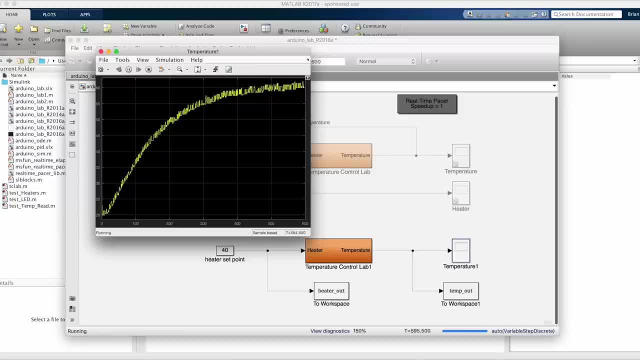 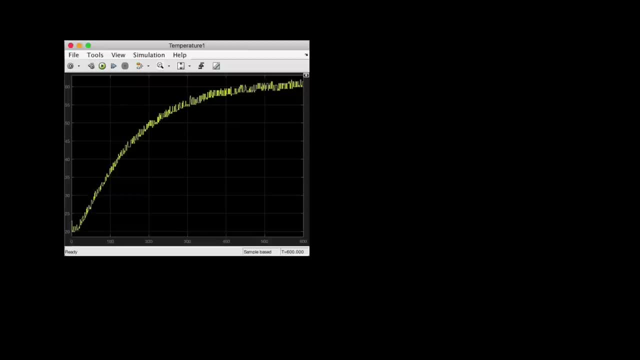 And that's nearly the same step response that we saw earlier, except this time with a heater set point of 40%. I'm going to try to approximate this system with a first order transfer function. We'll need to include a delay term or dead time as well, since we already know that there's delay in. 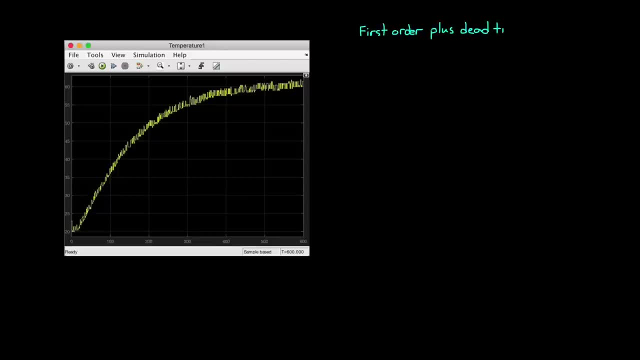 the system. A first order plus dead time transfer function requires three things: the gain, the time constant and the delay. The gain can be found by dividing the rise in temperature by the rise in the set point. The temperature went from about 20 to 60 degrees and the set point went from 0 to 40%, so the gain works out to be about 40 over 40, or 1.. 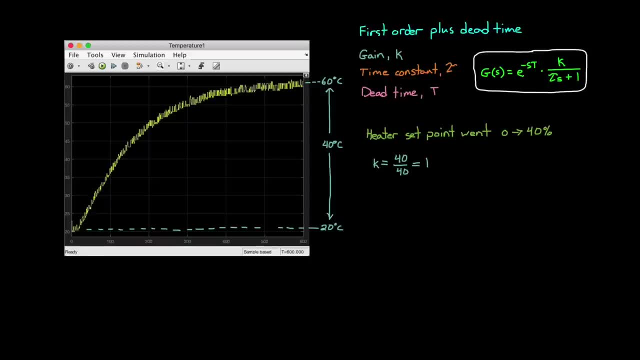 The delay term is how long it takes for the temperature to start rising after the step is applied. It's hard to tell exactly, but it looks to be about 10 seconds And the time constant is a measure of how fast the system rises. It takes about 5 time. 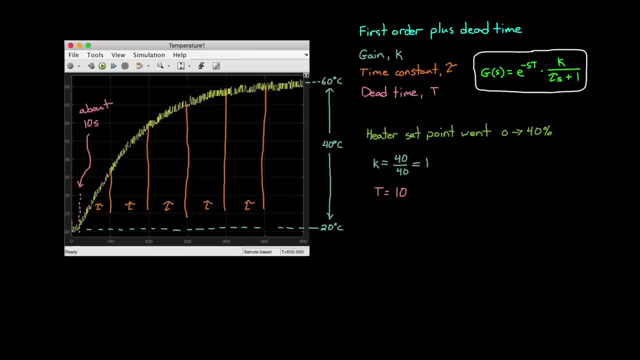 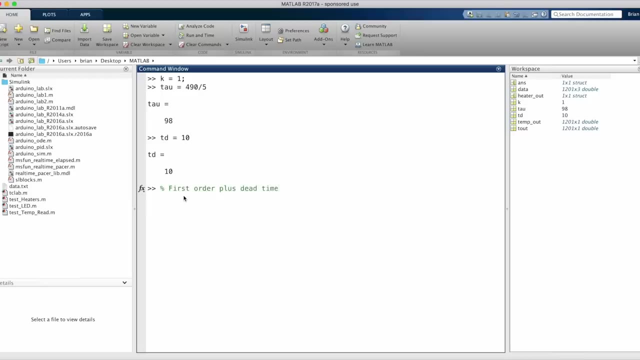 constant periods to go from 0 to 98% of the steady state value For us. it gets to steady state around 500 seconds. so minus 10 seconds for the delay and divide by 5 gives us a time constant of 98 seconds. I can use the tf command in MATLAB to generate the first order plus dead. 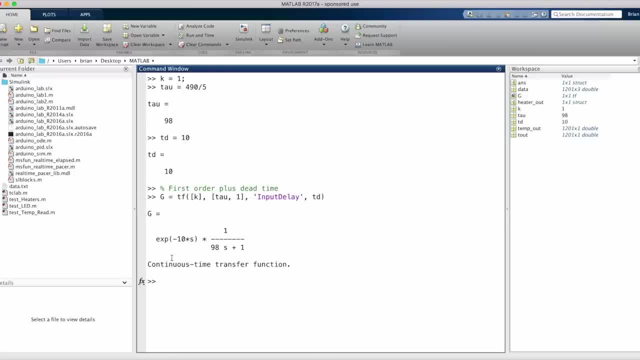 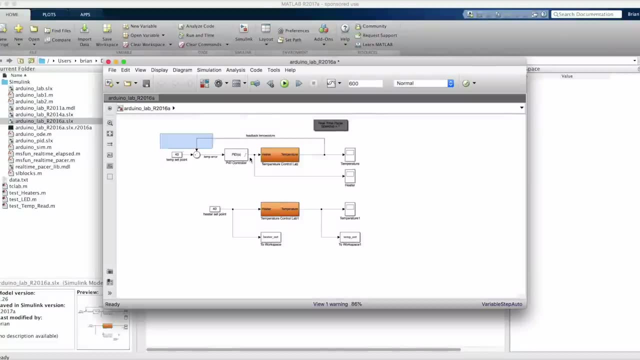 time transfer function And I get e to the minus 10s, which is the 10 second delay times 1 over 98s plus 1.. Or since I'm working in Simulink, I can just build it there as well. Now, this is just the dynamic. 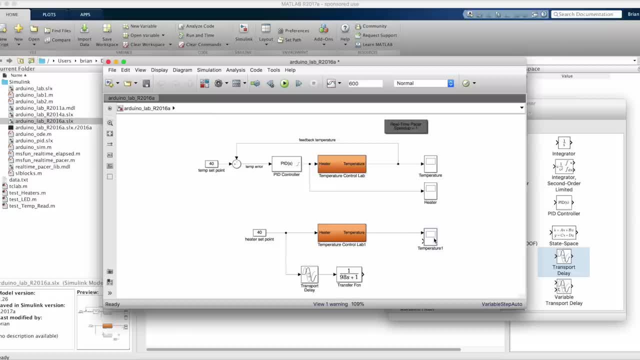 portion of the system and if we input it as 0 for the heater, the output of the system would also be 0 for this transfer function. But we know that 0 input means room temperature output, so we have to add a constant room temperature value to the output to create. 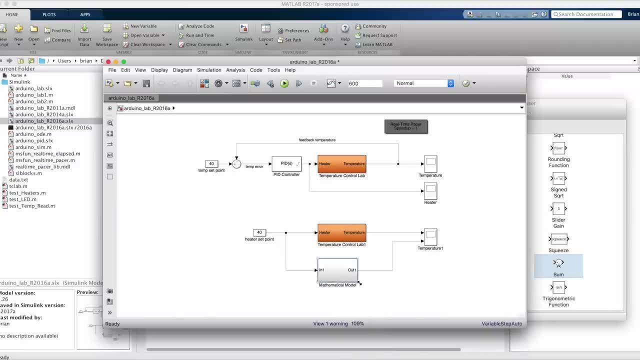 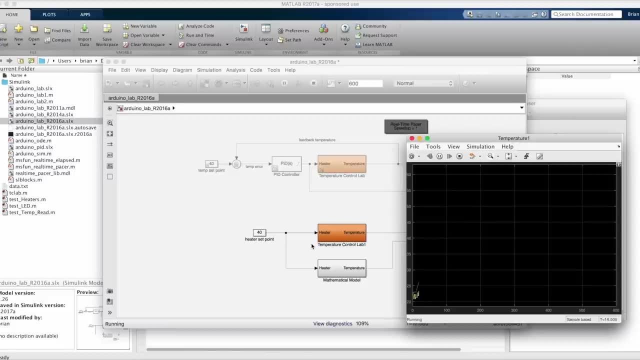 our mathematical model. And there we have it. Now I'll comment out the top system and run our model against the real hardware so we can see how well it does. Alright, I can see that it's running rising faster than the real hardware, so it's already a little bit off. But while it runs in, 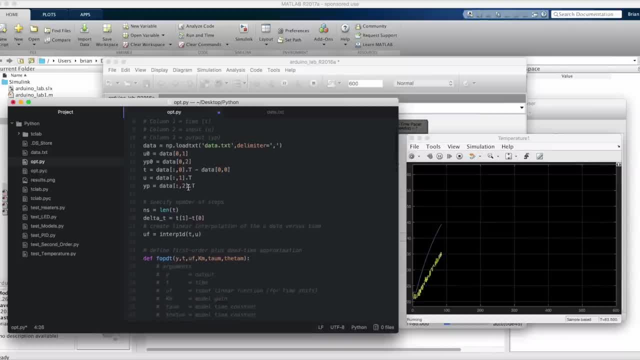 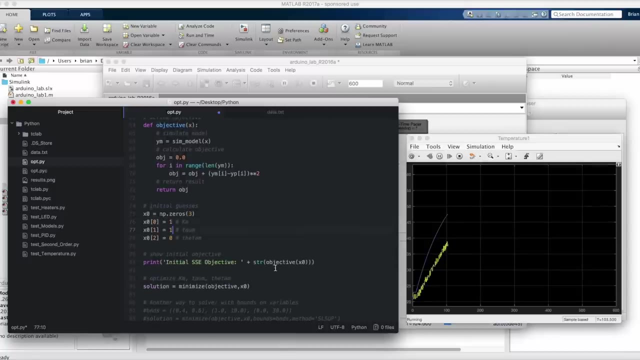 the background. I'm going to generate a better first order plus dead time model using a Python program from the AP monitor site that will find the optimal combination of gain time, constant and delay based on the step response values that I saved earlier. I'll set the initial guess to: 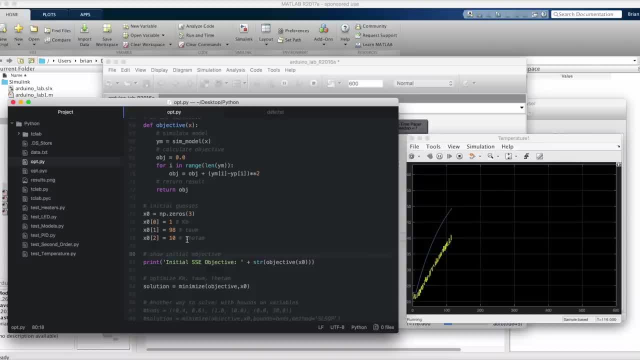 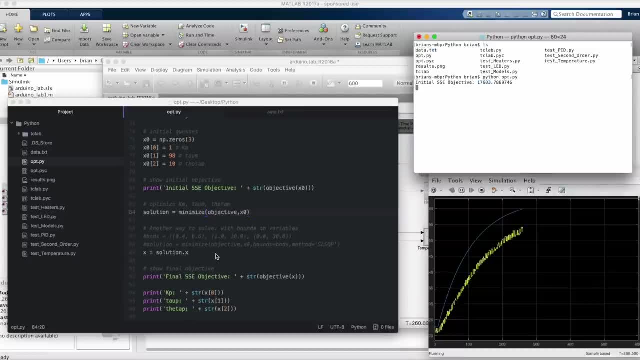 what I calculated by hand and then kick it off running. The script takes a three column data file, time, input and output, starts at the initial guess and then tweaks those values to minimize the sum of the squares of the error between the real data and the current model. 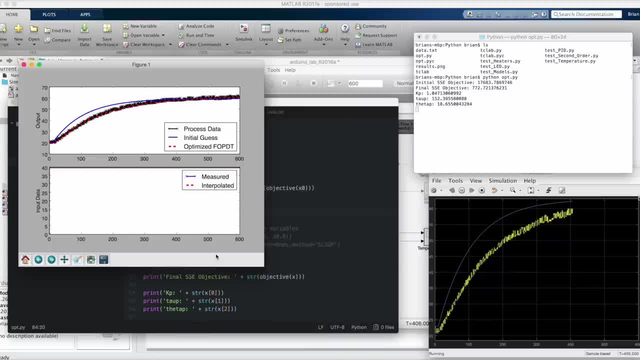 All right. now it's done. You can see the blue line, which was our original guess, rising much faster than our data, just like we see with what's going on with the test we're running right now. But the optimized set of parameters fall right on top of the test data and we can see the 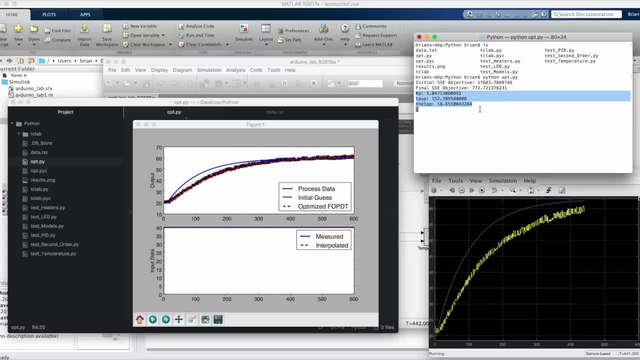 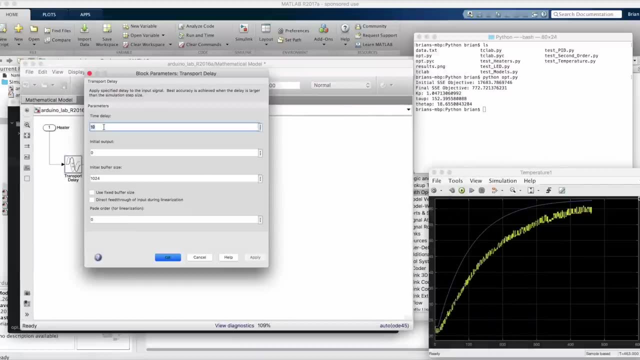 optimized parameters. in the script output The gain is 1.047, and the time constant is 152.4, and the delay is 18.6 seconds. And now we can go back to Simulink and change these parameters to the optimized ones. We'll have a much better first order model of our system with these parameters. 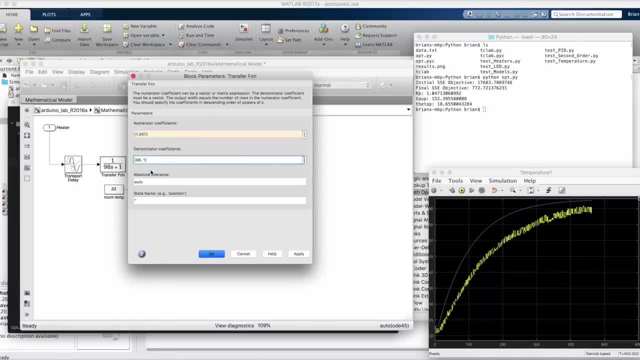 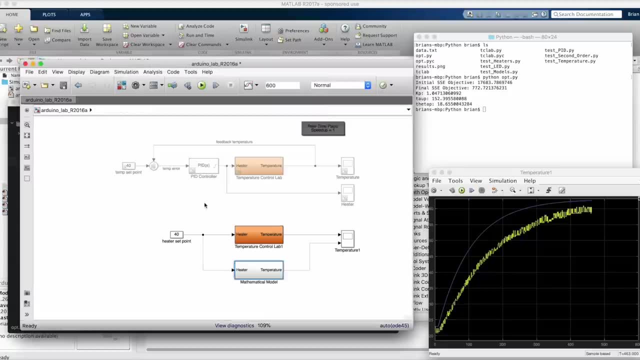 Now, at least for a while, we don't need our hardware to design a controller. We can use this new model to perfect our PID controller, try some feed forward control or build an optimal model predictive controller, And we may find later that the first order model doesn't accurately. 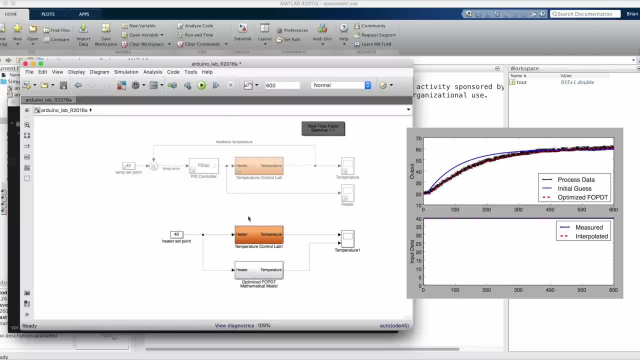 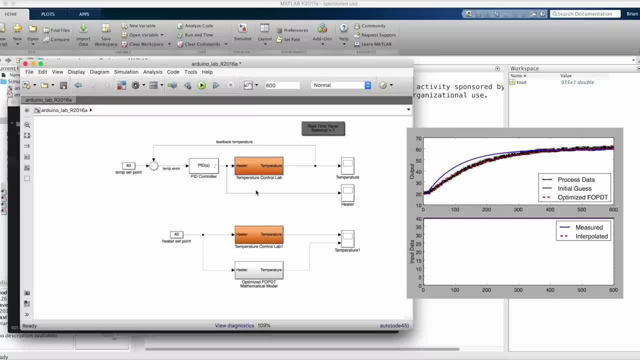